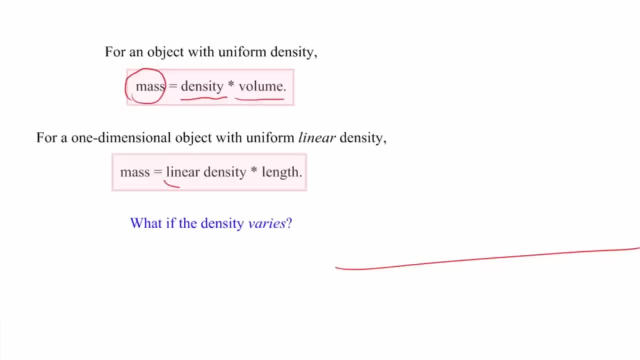 you know a rope or a wire or something like that, then the linear density, that's the amount of density, just because it's one-dimensional, we call it linear times. the length gives you the mass, And so if we want to, you know, 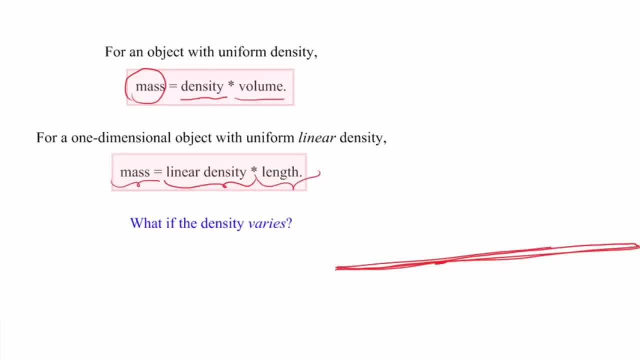 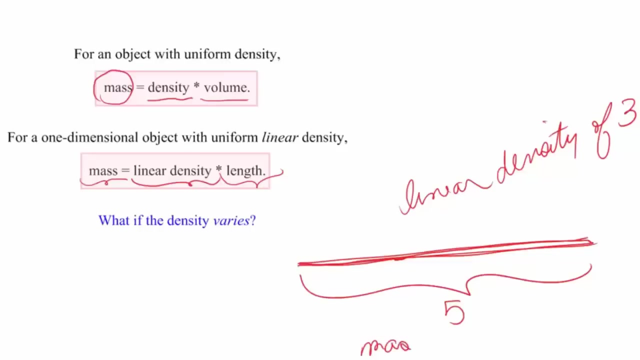 you know, for example, you have say: you have this piece of wire here, it has a linear density of 3, and it has a length of 5, then it could have a mass of 3 times 5 or 15.. Now that was. 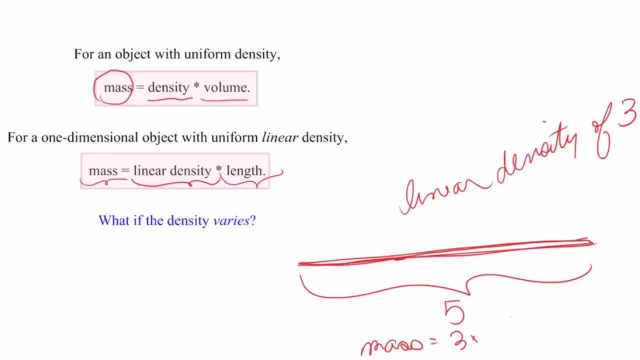 really basic and without even worrying about units, but that's kind of the idea. Now where the calculus comes in is: what if the density varies? What if the density right here for this, at this point on the rod, is not the same as the density over here? at this point, How can we find the total mass? 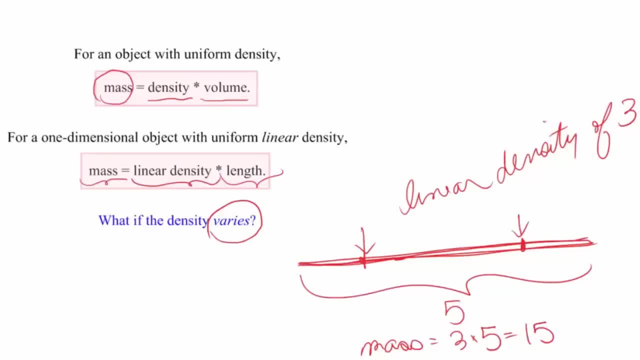 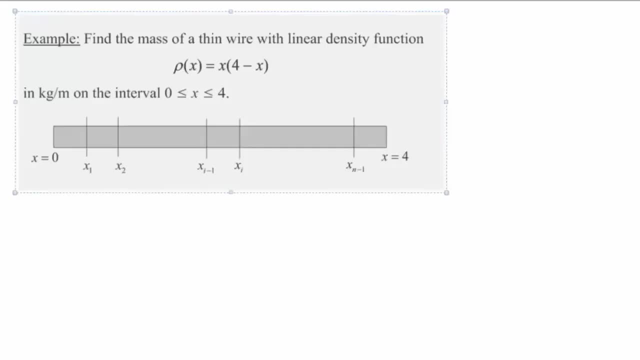 if we don't know, you know, if the density is changing. And what we're going to do is we're going to do calculus, We're going to take this rod and we're going to slice it up into itty bitty, little thin slices. 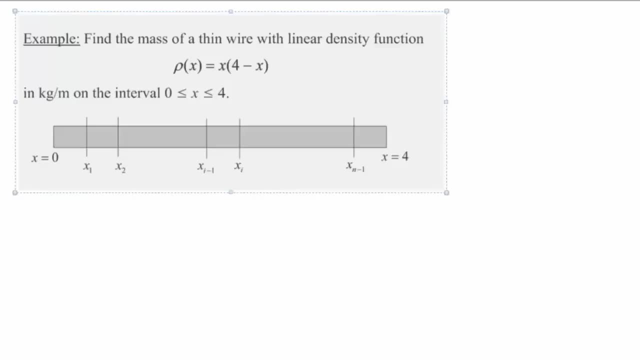 And in every slice. you know this is the slice here at the point XI, and it's right. here we're going to take this little chunk out. it's going to have a width of delta X and on that little chunk we can assume that the density's constant, So we can plug in. 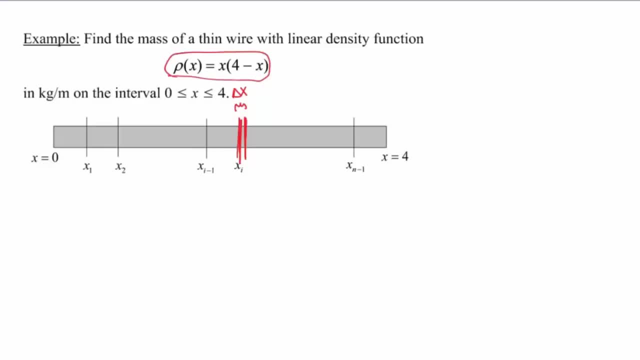 our X value into our linear density function and if we take our X value there, which would our X value there, which would be X for minus X, and we multiply by our delta X the width of our little slice, then this is giving us our density times our length. and what does? 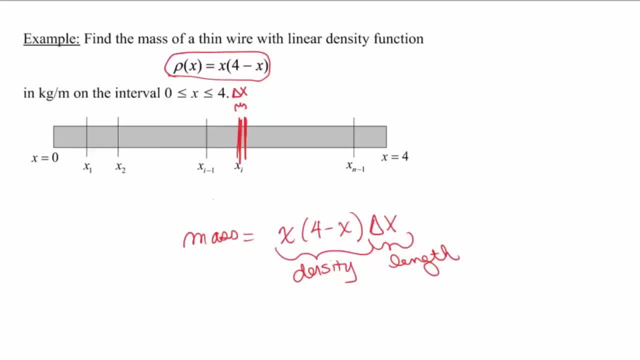 that give us. That gives us mass, but that's only mass for one little slice. If we want the mass for the whole thing, we're going to have to add them up, and the easiest way to add up a bunch of infinitely thin little slices is to integrate. 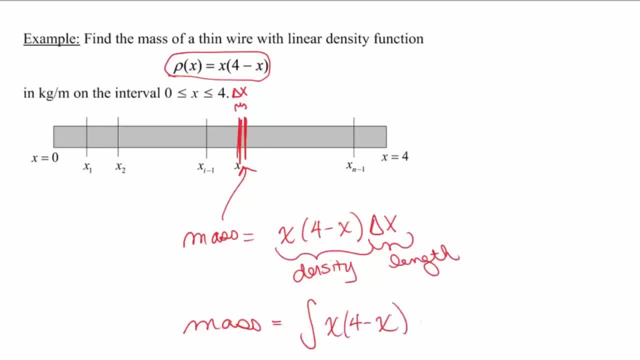 We're going to integrate our density function and then our delta X turns into a DX when it gets infinitely small from zero. if that's where we want to start here, that we call that X equals zero up to wherever the rod ends, and that's going to give us our mass. 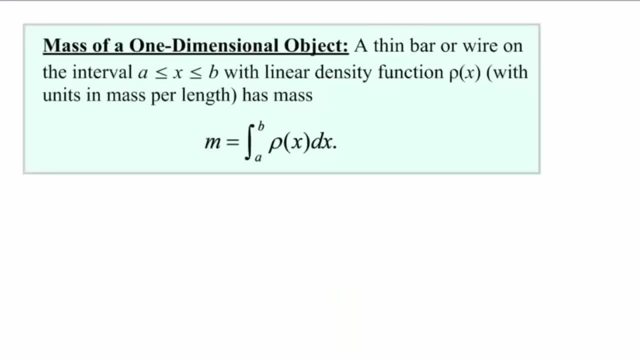 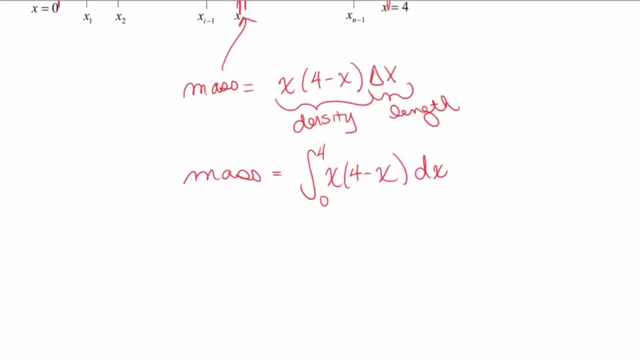 Let's do this. This is what we just said. right, Rho there stands for density. so we've got our density, We're going to integrate it and it's going to give us our mass If we do this example we've got here. how would we actually do that? 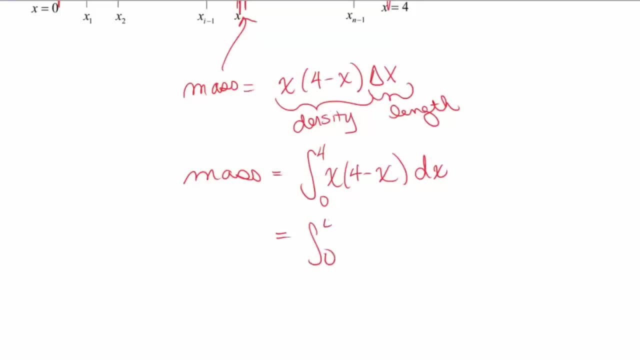 Well, if we wanted the actual mass, we would have to FOIL this out. then we'll do our power rules, We'll take our answer and we'll plug in using the fundamental theorem of calculus. so we'll have 2, 4 squared, minus 4 cubed over 3, that's plugging in 4, minus when we plug. 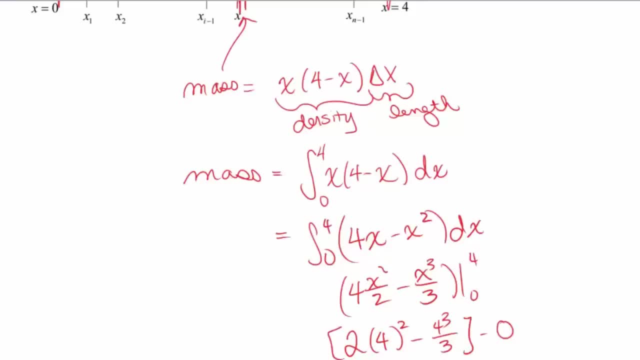 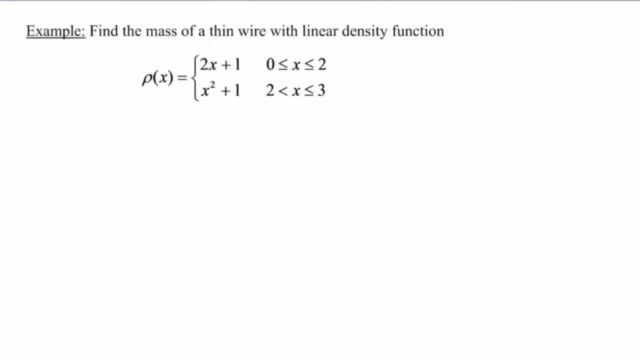 in zero. we're just going to get zero, and that's our mass. That's linear density. Here's another example. it says: find the mass of a thin wire with the following linear density function: This one's a little bit funny, because our wire here 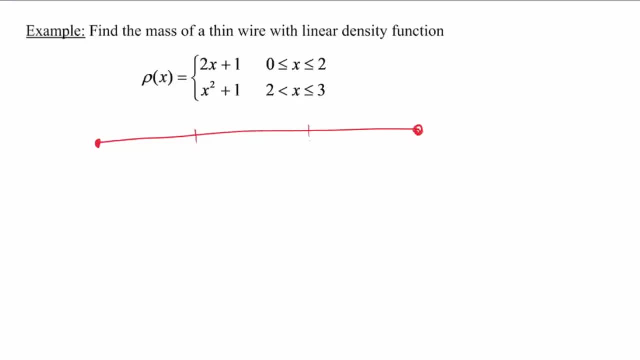 It's three units long, one, two, three, but for the first two the density function is 2 X plus 1, and for the last part here the density function is X squared plus 1.. We're going to deal with this the same way we deal with piecewise functions normally. 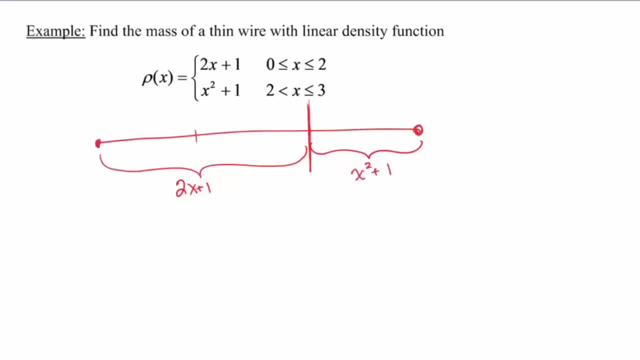 or physically. we can think of it as almost as cutting this wire and finding the mass of each piece and then adding them together. Our total mass here It's going to be the integral from zero to two of 2 X plus 1, plus the integral from. 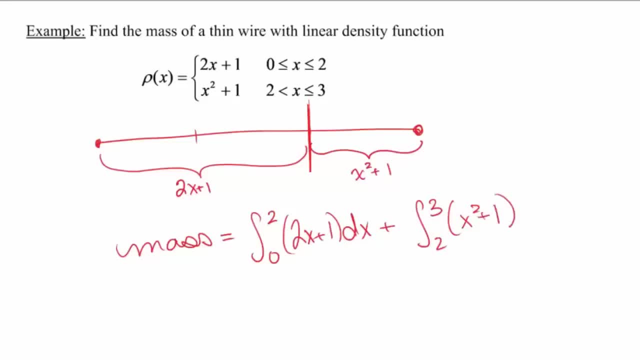 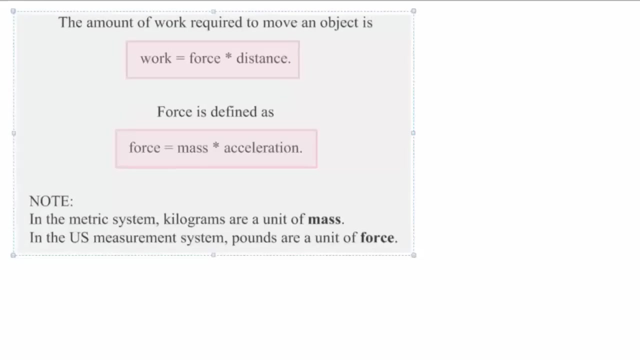 two to three of X squared plus 1.. All right, the next application we're going to talk about is work. This is a physics concept. Work is the amount of- You know The amount of, I guess- work required to move an object. 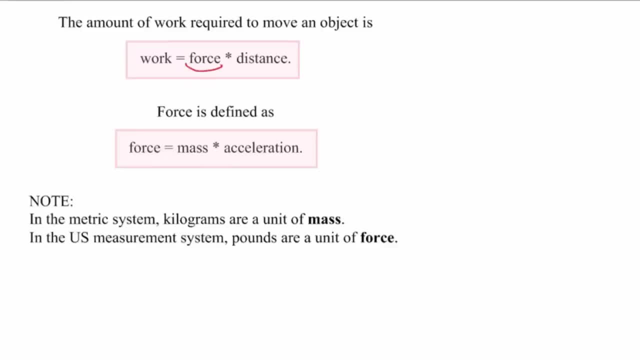 What that is is you're going to take how much force you have to use to move that object and multiply it by the distance that you move that object. That's the total amount of work that you spent. Force is defined as mass times, acceleration, and then we just talked about mass being volume. 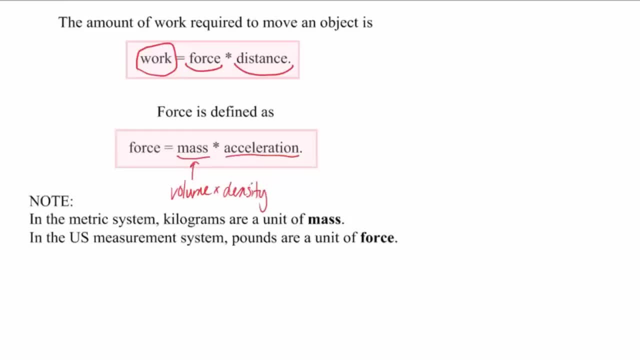 times density. Okay, If it's a 3D thing, If it's a 2D thing, it would be area times density, the single dimensional things. The lines we just did were length times density, All right. so if we want to find the total work we're going to end up probably doing, 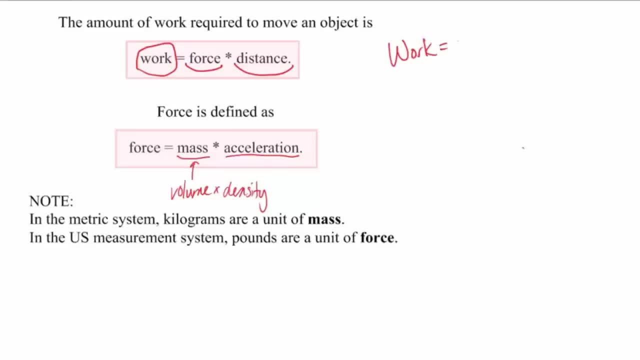 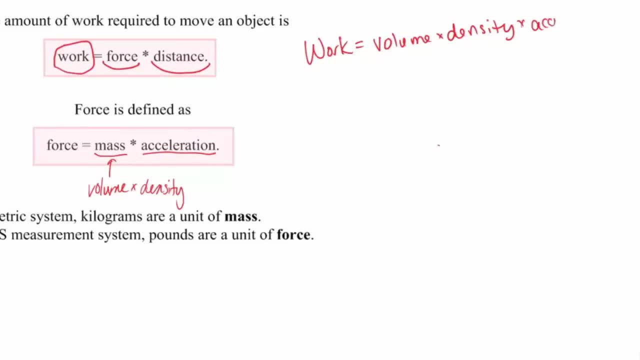 something like volume times density to give us mass times acceleration. Okay, That's the total work we're going to end up doing. We're going to end up probably doing something like volume times density to give us mass times acceleration, To give us force times distance to give us work. 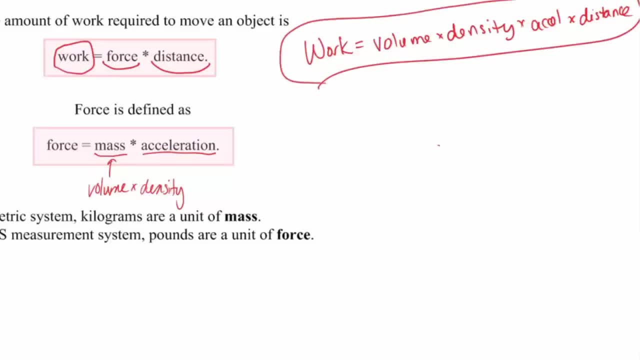 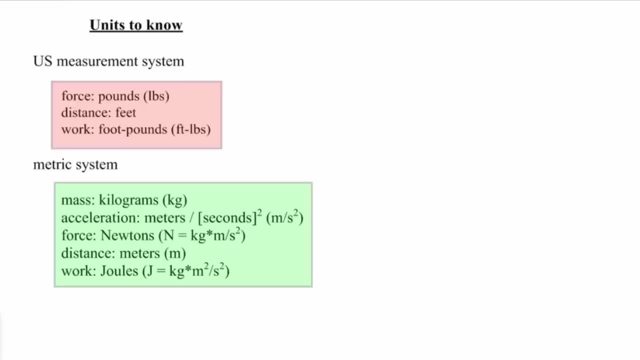 We're going to end up doing all those things together if we want to find work. A couple of things to know about work is that the US measurement system and the metric system are a little bit different here, because for the US we have a measurement for force. 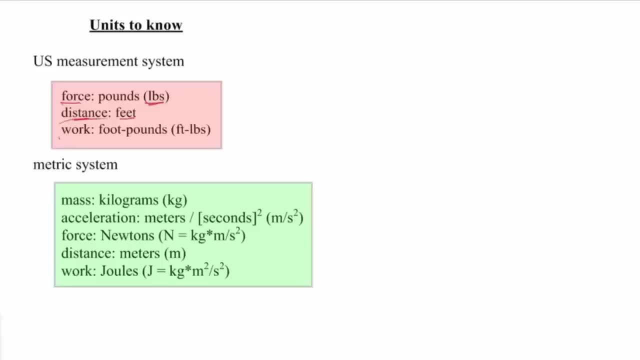 It's pounds. Distance is feet, Then work is measured in foot Pounds. That is number of feet times number of pounds. In the metric system they don't have a unit that's for force. they have a unit for mass. 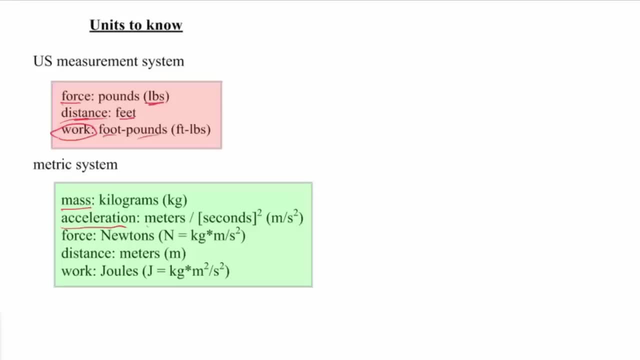 That's kilograms. Then you have to multiply it by the acceleration to get the meters. This is usually what they give you is the kilograms and the meters. There is a force here, newtons, but usually they don't give you a problem. statement in. 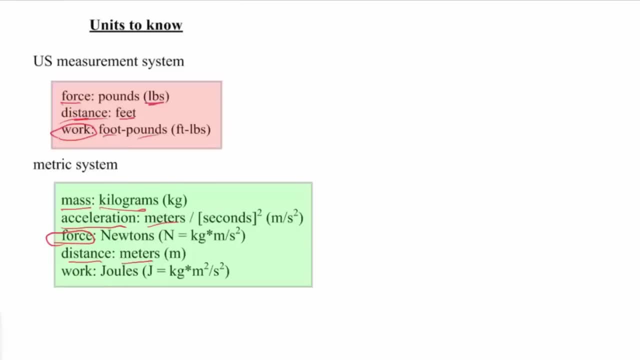 newtons, Then you have to make sure your distance is given to you in meters as well. The total of the work here is in joules. Whenever you're doing a problem, before you start make sure all your forces are in pounds. 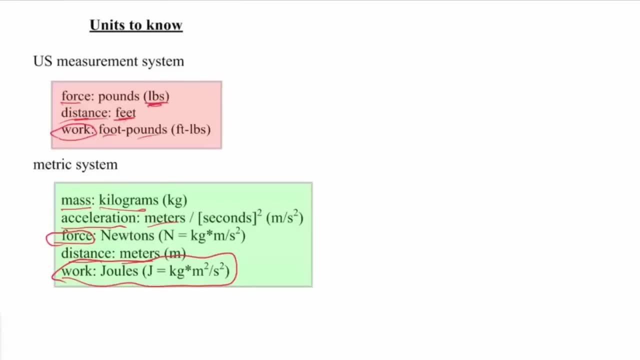 all your distances are in feet. so if they give it to you in inches, convert to feet. That will give you the work in foot pounds for the US system. Or if you're in the metric system, make sure your mass is in kilograms. your acceleration: 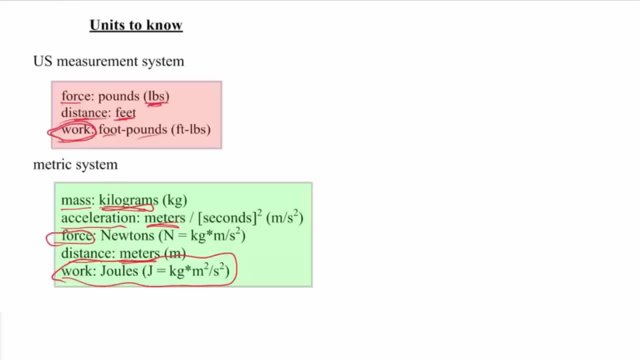 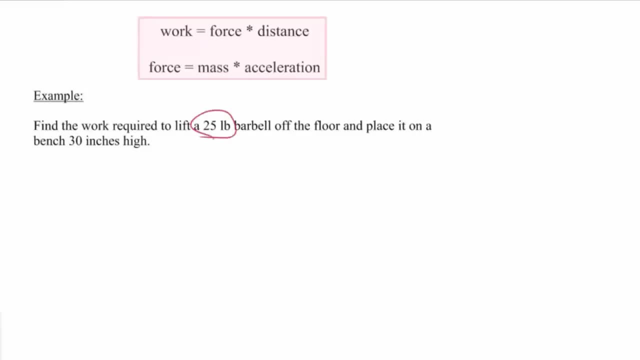 is in meters and your distance is in meters, and then everything else will work out. An example of work This is: find the work required to lift a 25 pound barbell off the floor and paste it on a bench 30 inches high. 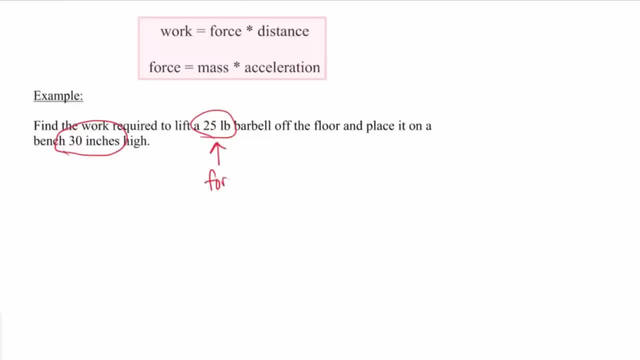 The 25 pounds, that's our force and the 30 inches, that's our distance, except remember, the distance has to be in feet. so 30 inches is 2 1⁄2 feet. The way you find that is to say 30 divided by 12, because there's 30 inches and 12 inches. 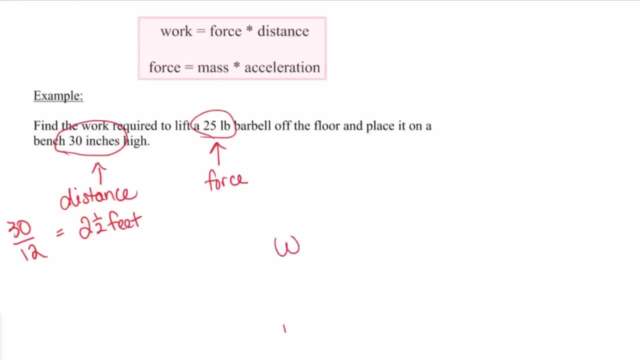 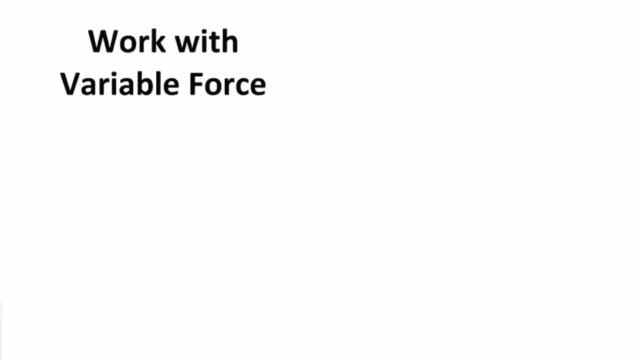 in one foot. Now how much work is it? The work is going to be the force 25, times the distance, 2 1⁄2, to give you 62 1⁄2 foot pounds as your work. 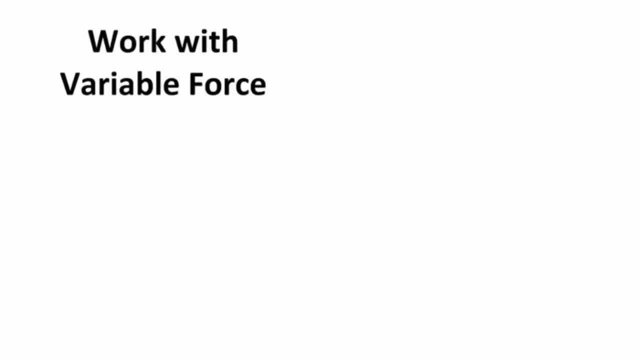 The calculus comes in again when you have something that's not consistent. It could be that the force is changing, it could be that the distance is changing, or it could be both. The first example here we're going to have is going to be the force changing. 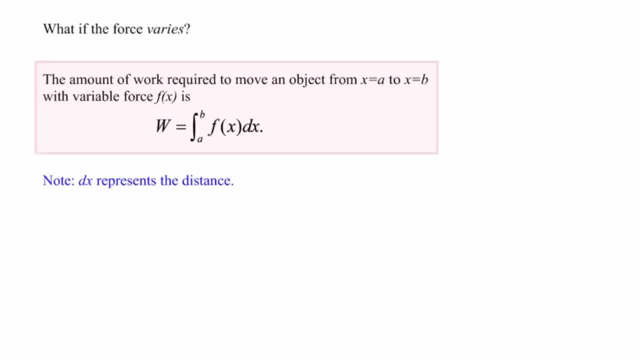 The force is changing, then we're going to do almost exactly what we just did with density: We're going to take our force and we're going to take whatever our thing is. we're going to chop it up in little bits and we're just going to go a distance of dx every time. 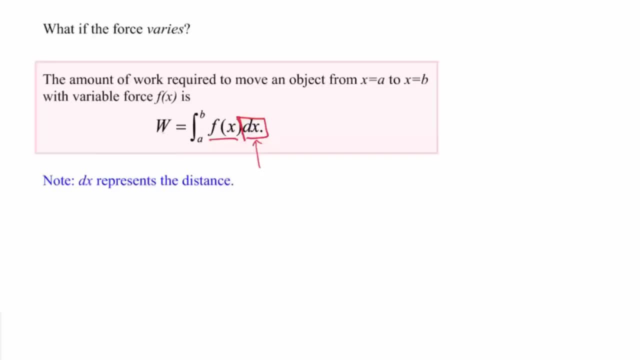 Then we'll add up all of those forces to get All of those little bits of work, to get our total work. We're going to have a little bit of work being your force at a particular point x, let's call it x. i bar times the distance of that little tiny section x and that gives you your little. 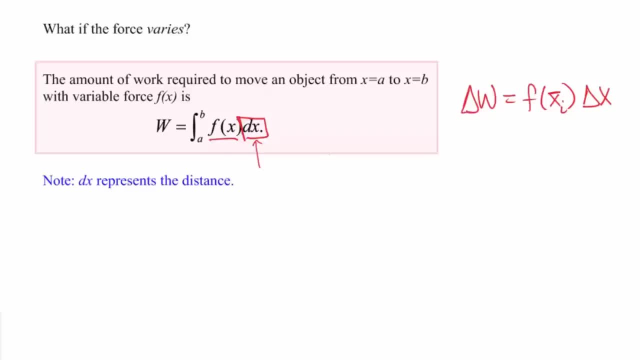 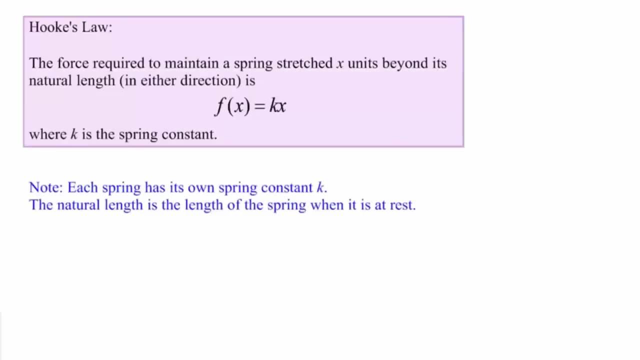 tiny bit of work and then, if you integrate this expression, that adds up all the work. Here's an example of that. This law is a law for spring. it says the force required to maintain a spring stretched x units beyond its natural length in either direction is f of x, that's your force equals. 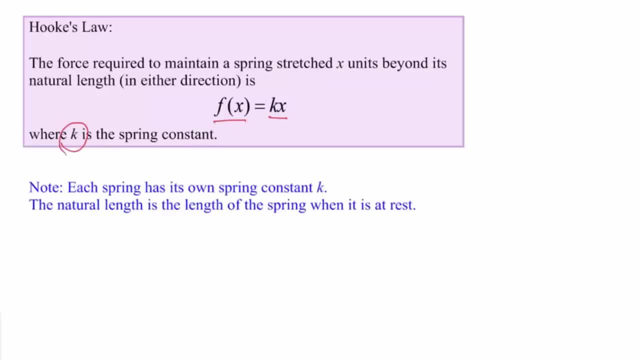 kx, where k is the spring constant. Depending on your spring, you're going to have a different value of k. You guys have played with springs before right. Some of them are stretchier, some of them are harder to stretch. 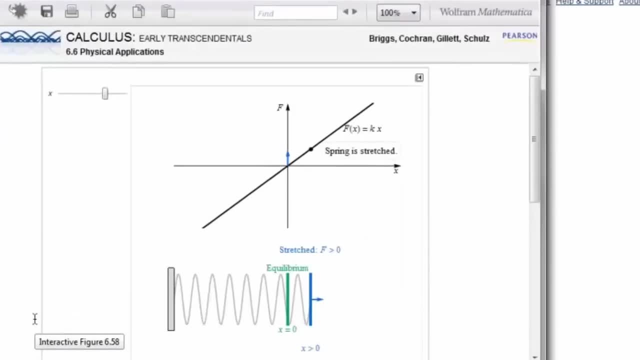 That stretchiness measure. that's where k comes in. There's our spring. Okay, If we put x right there, that's the equilibrium. What that means is that that's where the spring would be if you just set it on a table and 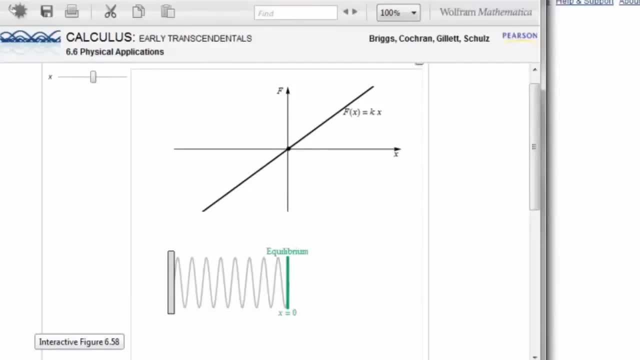 you left it alone. The work required to keep it there, the force you need, is zero. but as soon as you try to stretch that string, it takes positive force, and as soon as you try to compress that string, it takes force in the negative direction. in order to do that, 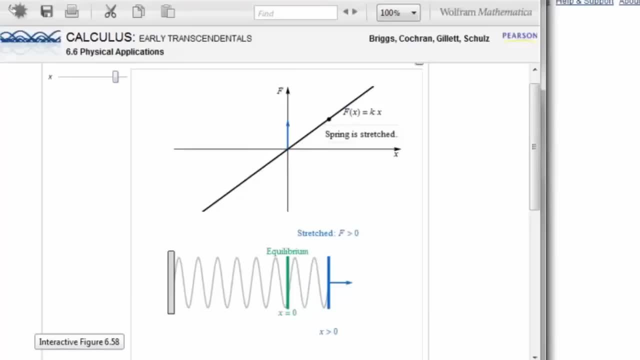 When we're trying to find out the work force, The work you're doing while stretching it or compressing it, that amount of force changes. It's easy to stretch it. when it's close to resting, it's pretty easy to stretch it. or? 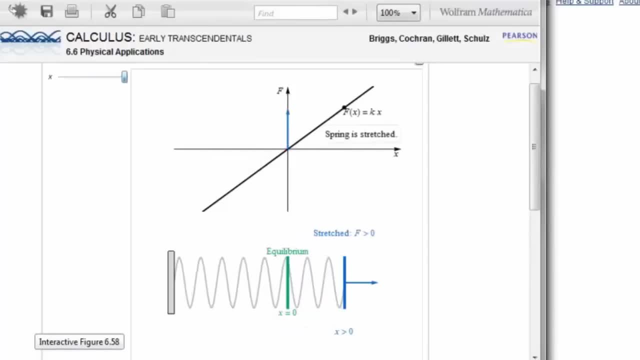 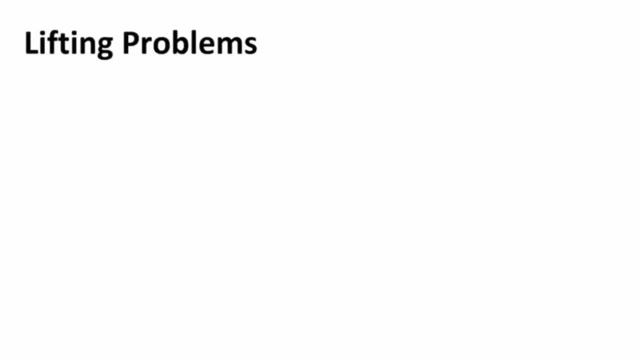 compress it, but when you get out farther away, it suddenly gets really difficult to stretch it anymore or really difficult to compress it even more. This is a lifting problem. Okay, For lifting problems. this is where distance is going to vary, because if you're lifting, 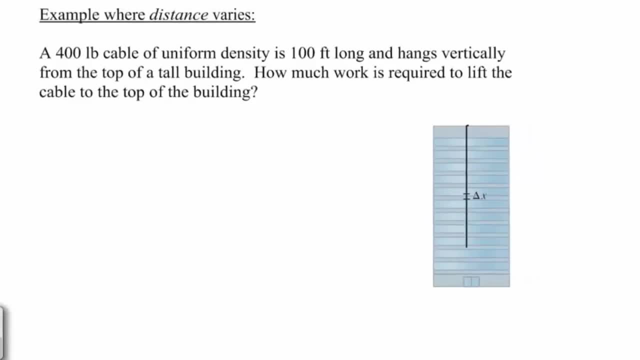 for example, here you're lifting this table up to the roof, then this little slice right here that they gave you, you have to lift it up this distance. If you took a little slice up here near the top, you barely need to lift that at all. 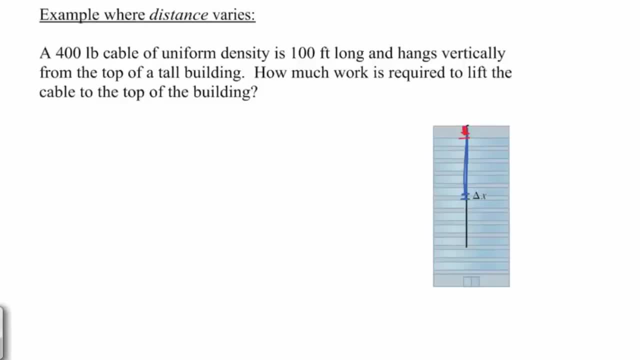 so that takes a lot less work. If you take a little slice down here at the bottom, you got to lift that the whole way, so that takes more work. If you're doing something like lifting up a cable, we are going to have to have distance. 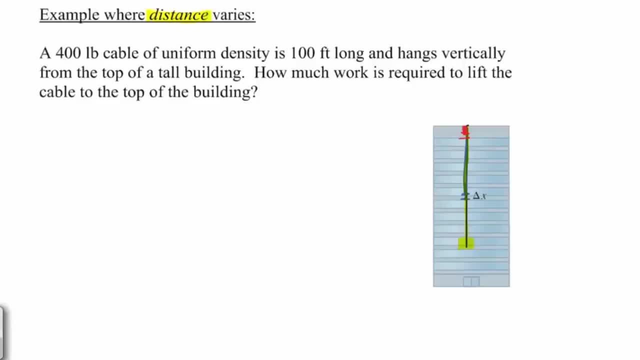 vary. How are we going to do this? We're going to chop it up into little segments like this, and on each little segment right there, we're going to be able to assume that for that little piece, the distance is the same. 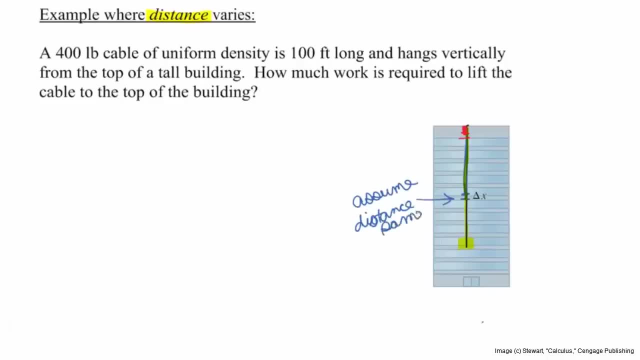 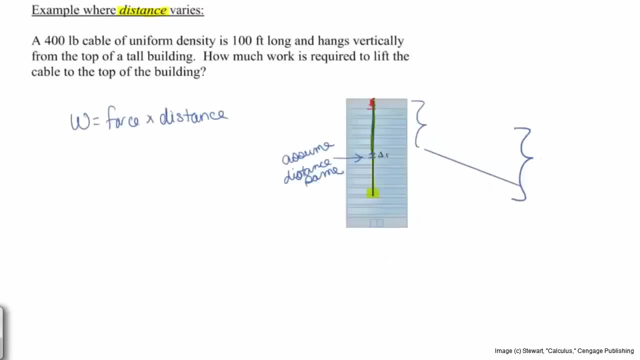 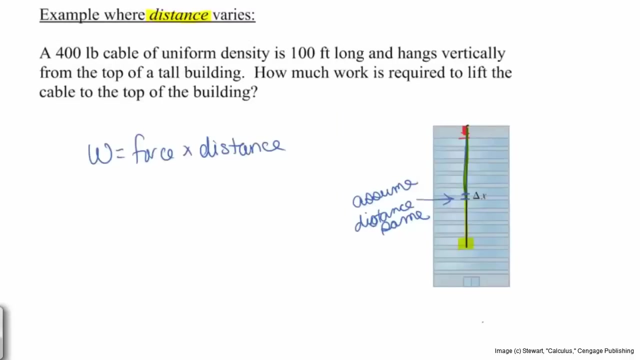 Okay, Okay, Okay, Remember, work is force times, distance. right, If we say X maybe is the distance from the top, so let's call this: X is the distance from the top, Then our distance will be X. Then we need to find the force. 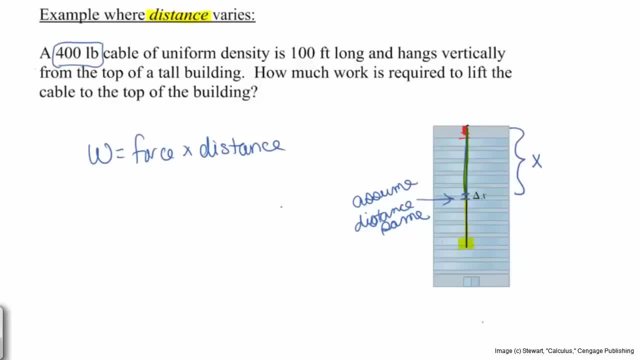 Now, the whole cable is 400 pounds, though, so if we're trying to find a little bit of work done on that little distance, delta X, the distance you're going to have to lift it up is going to be X. let's say that, and then how much is that little bit going to? 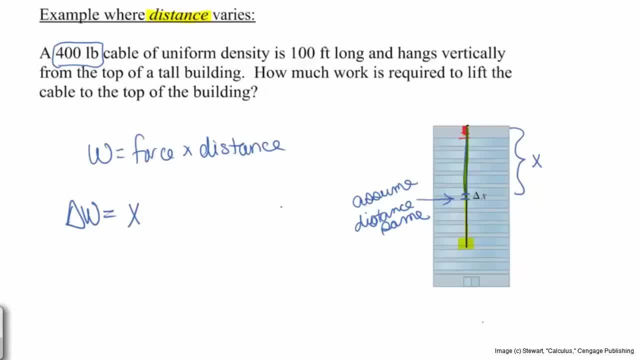 weigh Well, 400 pounds of cable is 100 feet long. That means that this cable is 4 pounds, 4 pounds per foot, and that would tell us that if we only have a little tiny delta X amount, then it would be 4 times delta X pounds. would be how much our little tiny bit there. 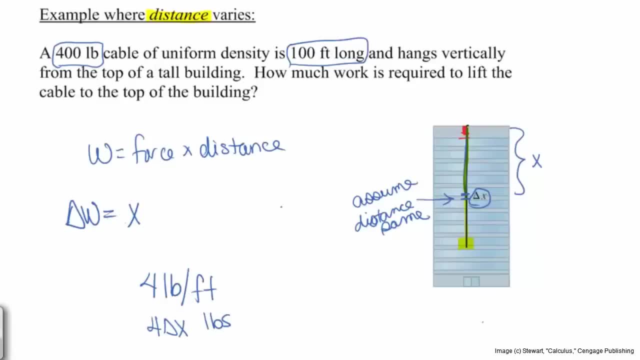 would weigh. Delta W, the little bit of work would be X, that's the distance times 4 delta X, That's how much the little tiny bit would weigh, But the number of pounds that little tiny bit of chain weighs. 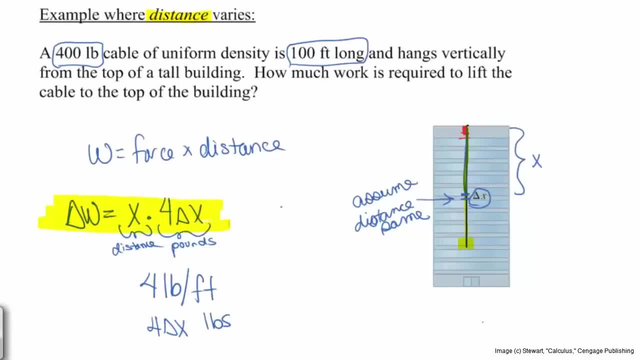 Now there's our equation for a little bit of force. Now we want to add up all those forces. so what do we do? We integrate. We're going to integrate for X and then, remember, the delta X turns into a DX. Then where do we start? 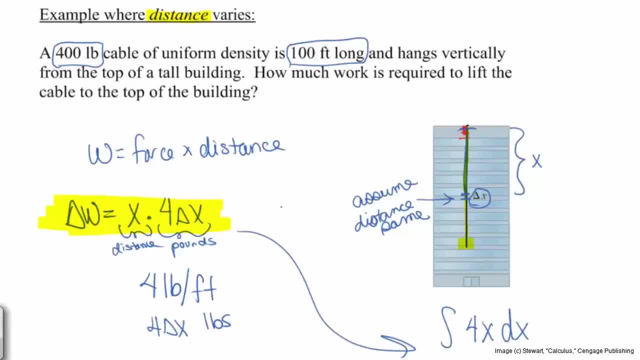 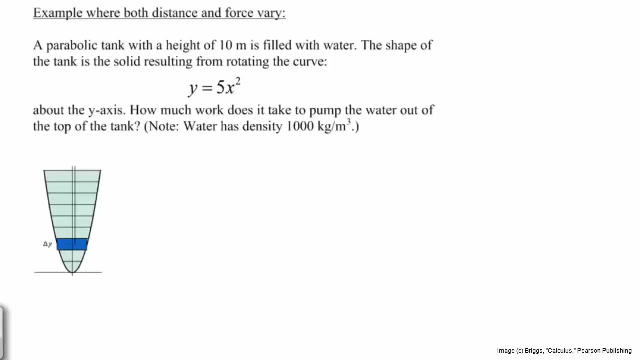 We start up here at the top where X is 0, and we stop when we've gotten the whole chain. That's down here. Then X is 100, and that'll give us the total work of picking up that chain. Our tank, shaped like this, is actually formed by revolving this parabola around the Y axis. 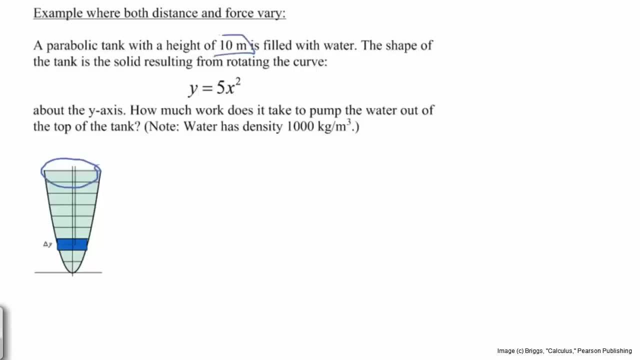 It has a height of 10 meters, so that means from here to here it's 10.. It's filled with water. The curve here that we're rotating around is: Y equals 5X squared. That's what we're spinning around. 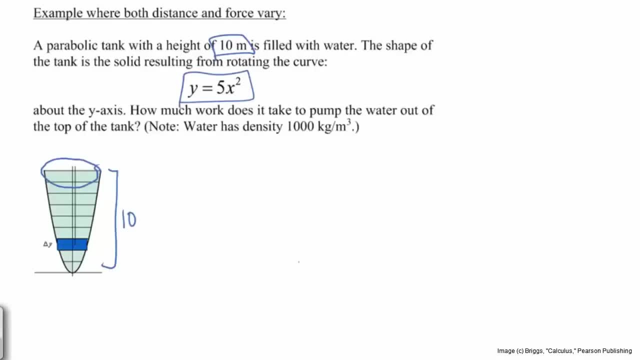 This is how much work does it take It takes to pump the water out of the top of the tank. If you look at this example, this is something where both distance and force are going to vary. Distance is going to vary because at each slice here, if we slice up our water each 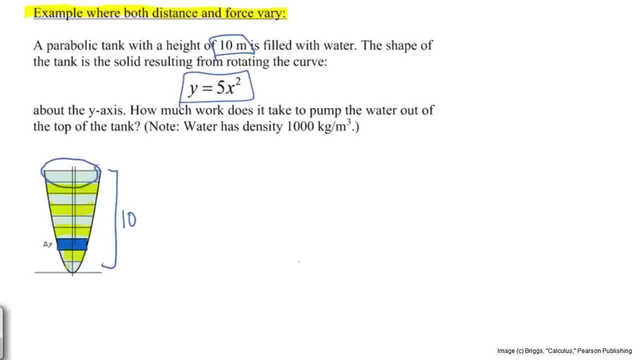 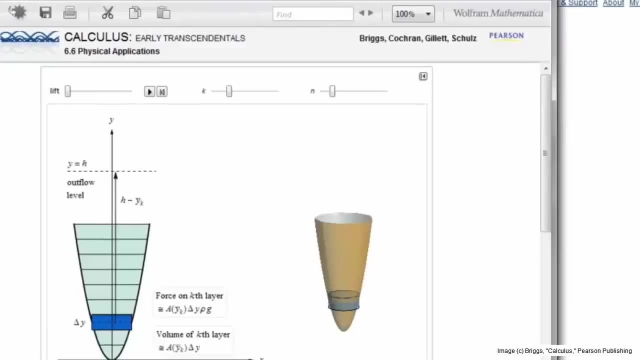 one of these slices has to go a different distance to get out of the top of the container. If I go back here to our book, we can actually look at a figure of this. There we are, There's our parabolic container. We're cutting it up into slices. 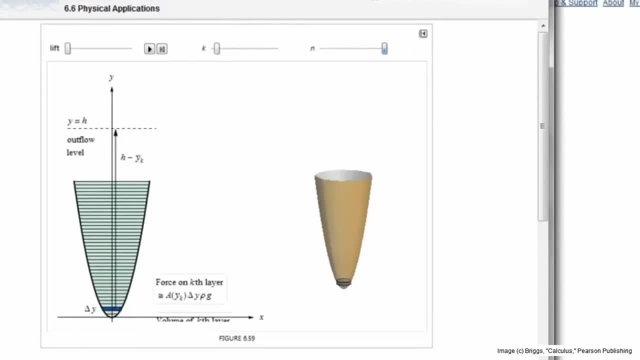 The more slices, the thinner it is, the closer it is to being exact, Then, depending on where your slice is. this slice is down here at the bottom. It's got a long way to go to get all the way out to the top. 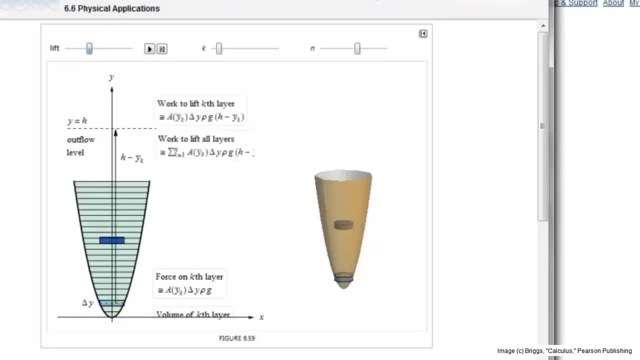 In this example they actually are lifting it up to above the surface of the container. I think our problem we're only lifting it right to the surface. Then we're going to imagine there's some kind of problem, There's a hose or something to take it away. 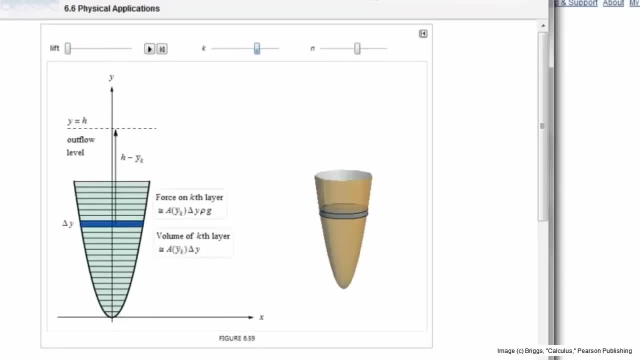 If we were to look instead at one of these higher up slices, that one, that's it. That's as far as it has to go to get out of the container. It hardly had to go at all. It's also important that where you take the slices are where the water is. 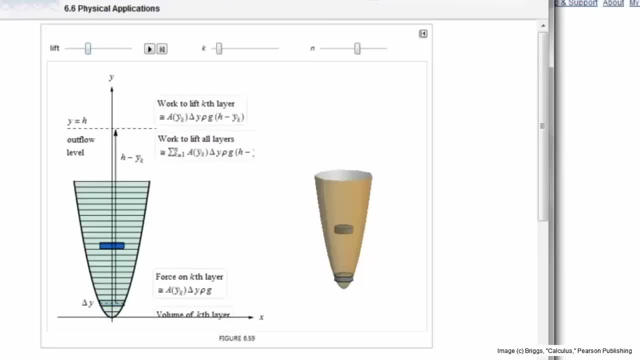 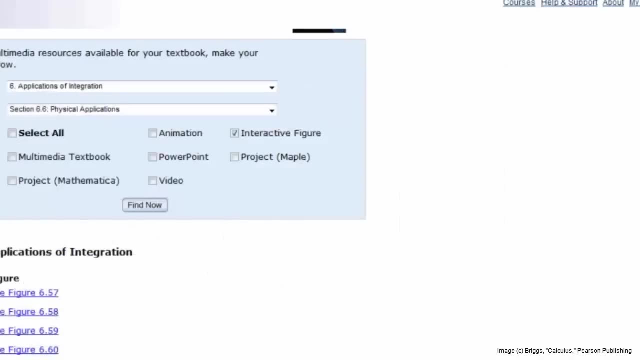 It doesn't matter the shape of the container. You start at the bottom of the water and you stop at the top of the water. Whenever we're lifting stuff up like this, we always slice it horizontally Right. Do it horizontally so that all the water in the same slice will have the same distance. 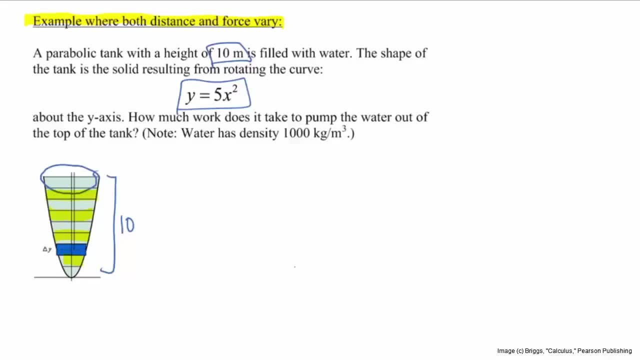 to travel to get to the top. Usually, when you do these, if they give you y equals 5x squared as your function, they're telling you already what your variables stand for. They're telling you that this way is x, with this being zero, and that this way is y, with 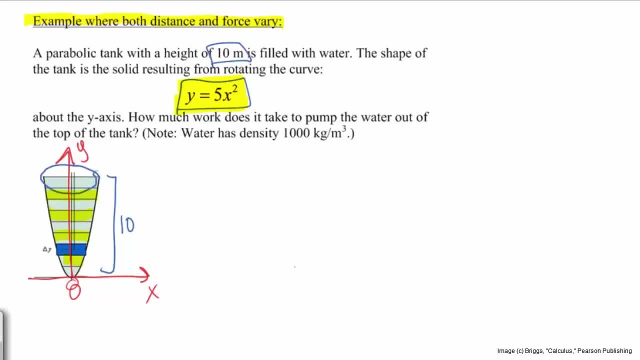 this being zero right here, The distance you're going to have to take. If this is your typical slice here, the one that's blue and the slice is at Y- just like when you're doing shells, your slice is at Y- To get from that slice up out of the top. 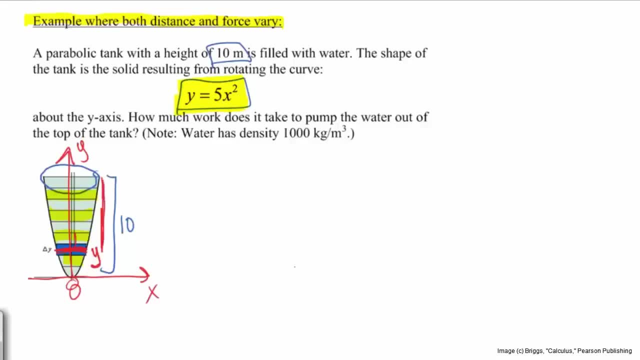 we need to go this distance right. That's the distance we want to find This distance from the axis up to our slice, that's Y, and the total distance is 10.. The distance our slice has to move is 10 minus Y. 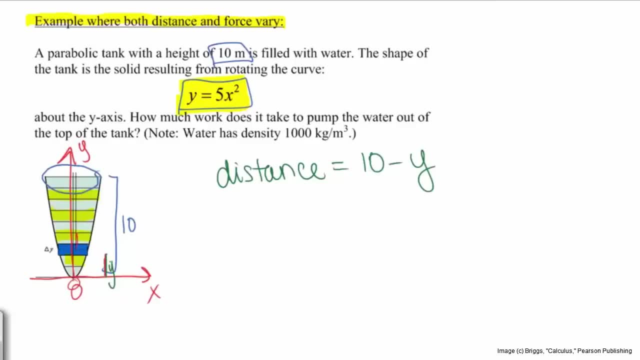 Once again that little green area that's Y. I've just made it red. This is what we want to find right here. We know that the total is 10, so if we take the 10 and we take away the Y, we get the. 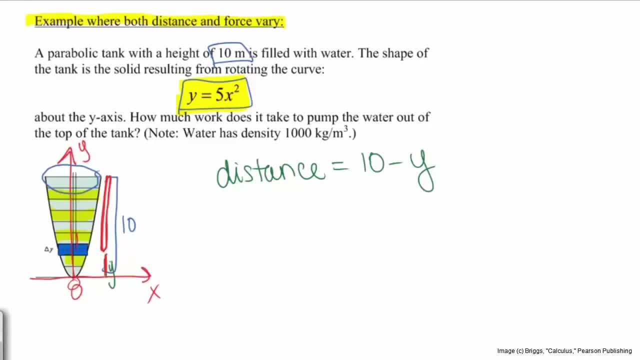 distance we need to go. that's 10 minus Y. The other thing we have to worry about is force, In this case, force. we are going to want to think of this as mass times acceleration. The acceleration is going to be the acceleration due to gravity. 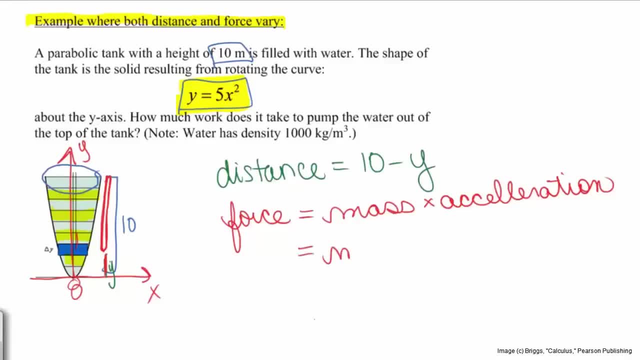 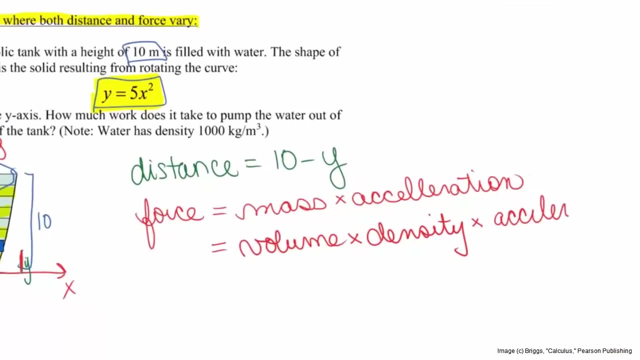 We're going to have to think of mass as volume times density. Lots of physics words going around here, but if you can just remember these formulas, how they go together, Okay, Then you can figure out which pieces you need for your particular problem. 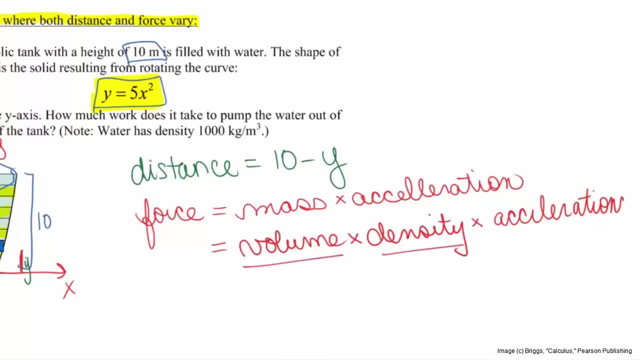 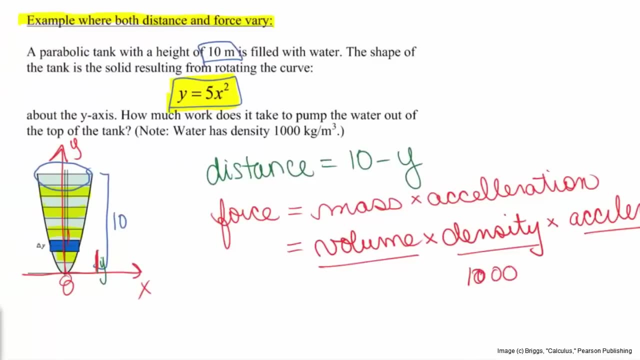 We need to find volume, density and acceleration. The good news is that they give you the density right there: it's 1,000.. Acceleration due to gravity is always the same: it's 9.8.. Now we just need volume. 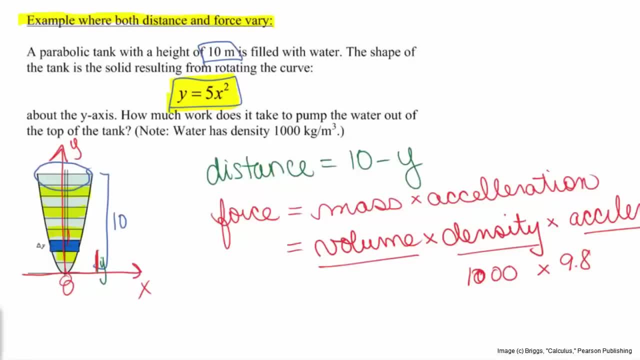 We need to find the volume of one of these little slices. The volume there is going to be the area. The area of that little slice times the thickness. The thickness is delta Y. The area that's a circle right. This is a disk. this is like the disk method. 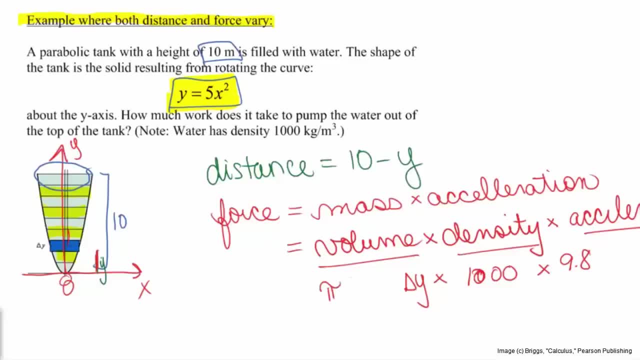 The area of that circle is pi radius squared. The radius is determined by the function. Right there, that red distance, there, that's the radius of our disk. The radius is the function. The radius is the function, That's our function. 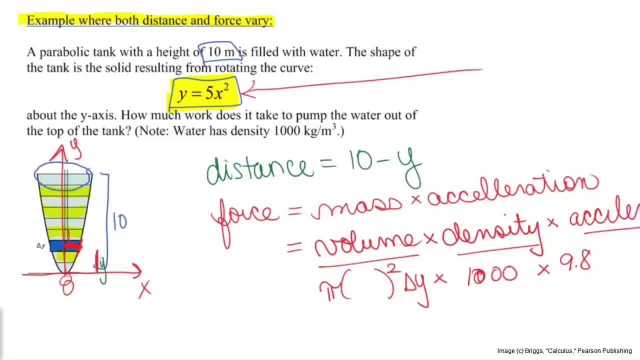 Our function is: Y equals 5X squared, but since it's horizontal, we need to solve this for X. X is going to be square root of Y over 5.. All right, so that's the amount of, that's the little bit of force it's going to take. 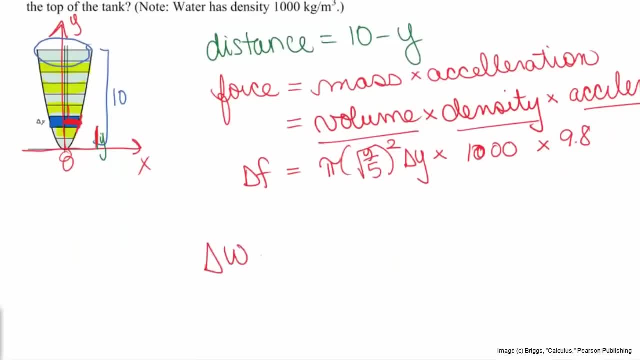 That means our little bit of work, for that one slice is going to be pi, square root of Y over 5 squared. Okay, Delta Y, that's our volume times 1,000, that's our density times 9.8, that's the acceleration. 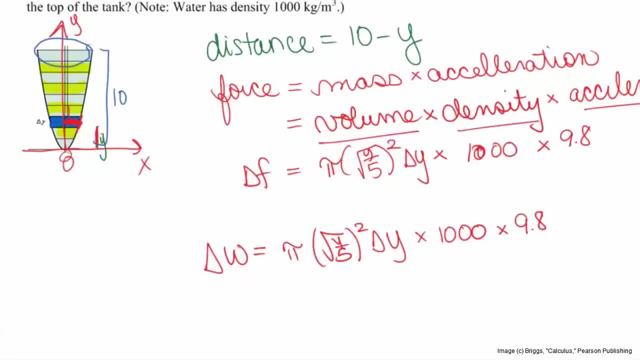 due to gravity. All that together gives you the force times 10 minus Y. that's the distance it has to go. Then, to add up all of those little pieces of work, we integrate, We get pi. I'm going to put all these constants together. 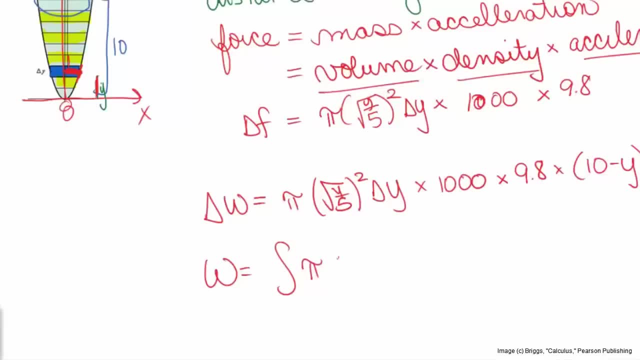 1,000 times 9.8, that's 9800.. Practically that's 9.8.. That's 9.8.. That's 9.8.. In fact, usually we write the pi afterwards, so we'll say 9800 pi, and then we have 10. 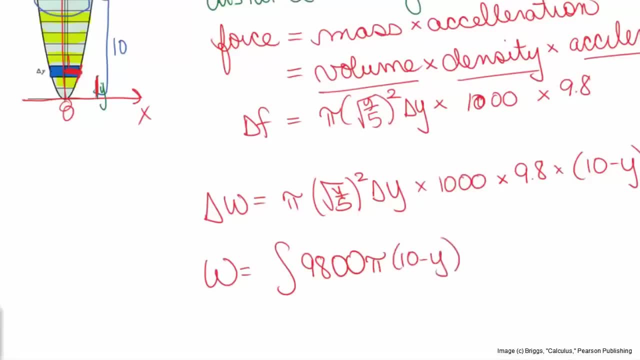 minus Y, square root of Y over 5. squared is just Y over 5, and then the delta Y becomes DY. There's our work. and where do we integrate from? Well, Y starts at zero. that's where we're going to start slicing. we're going to slice. 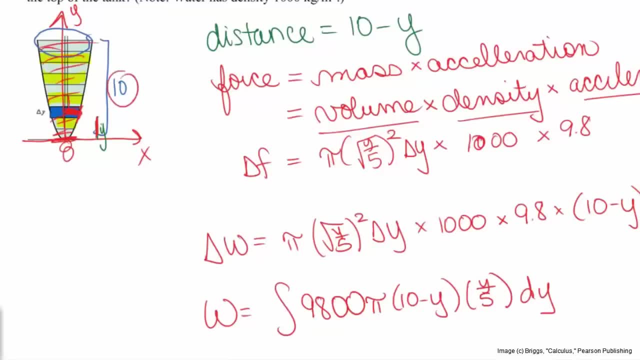 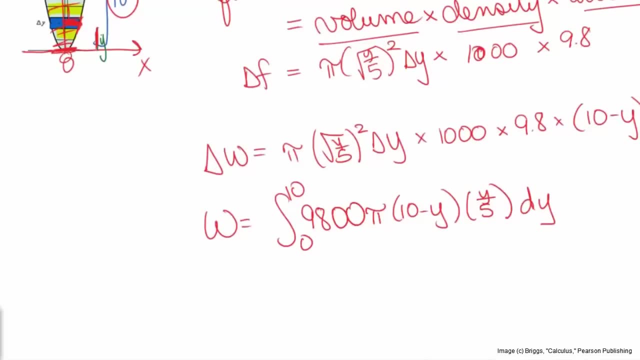 all the way up to the top, which is 10.. Okay, We're going to integrate from zero to 10.. Now this looks like it's very complicated, but remember that when you go to integrate, you can just pull those constants out front. 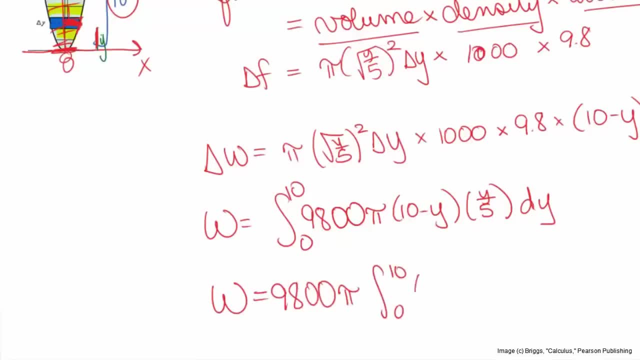 This integral actually isn't really much more complicated than a lot of them you've worked on before. In fact, you can even pull that five out front and there you are To solve it. you have 9800 pi over 5, times 10.8.. 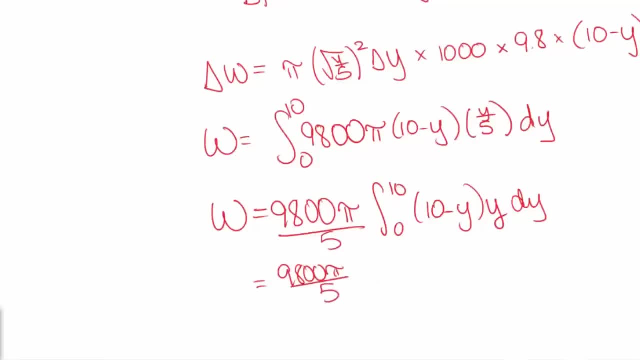 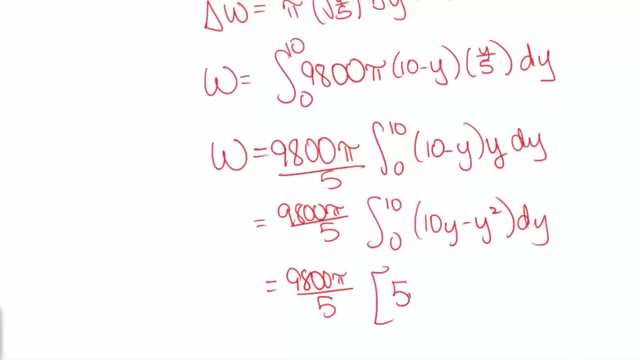 All right, All right. We're going to multiply that by 10 times the integral, from zero to 10, of 10Y minus Y squared DY, which is using the power rule here: 5Y squared minus Y cubed over 3, from zero to. 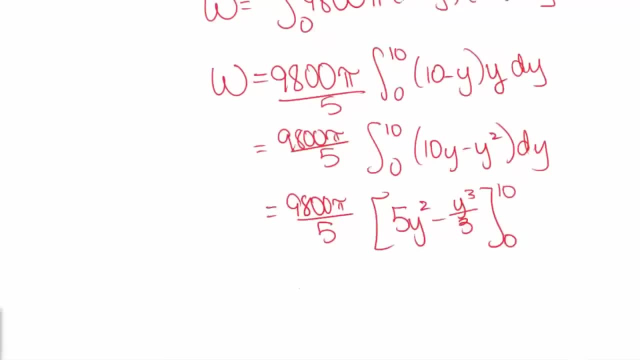 10, which is when I plug in. I've got to remember that these constants get distributed to all of it, so I need some big parentheses: 5 times 10 squared Minus, 10, cubed over 3, minus. when I plug in zero, I'm going to get zero. 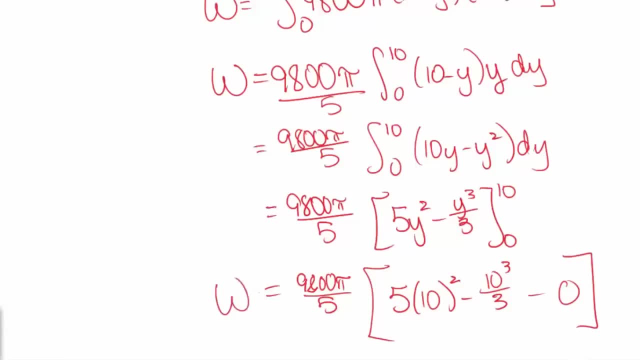 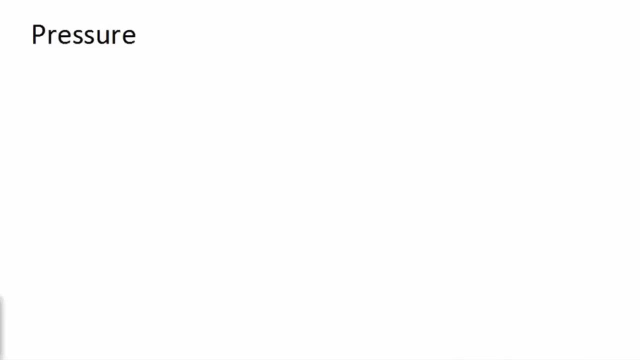 There we are. That's our work. The very last kind we're going to talk about is pressure Pressure. in particular, we mean hydrostatic pressure. That means pressure of water, still water. Pressure of water on the side of a swimming pool. 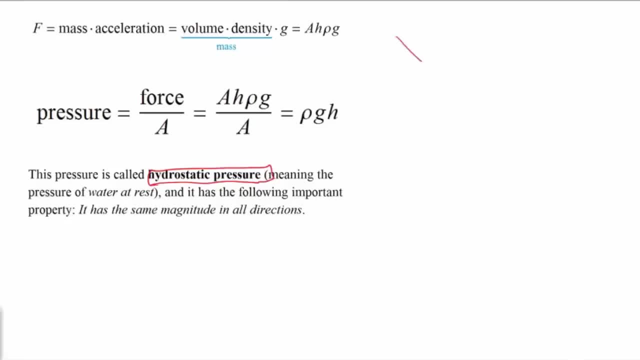 The book explains. it says: if you're in a pool and you're standing on the bottom and you can feel the pressure of all that water right above your head, that's hydrostatic pressure. If you're in the wall here, the wall also feels that pressure. 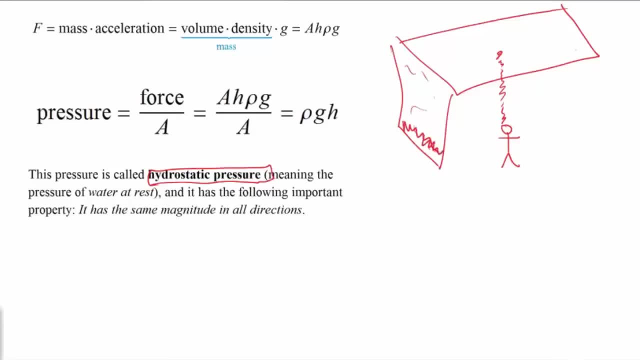 You can imagine, the pressure is heavier down here than it is up here, so if you're building a pool, you better make sure it's very strong down there at the bottom. Another example of where this happens a lot is a dam. so if you have a dam, here's your. 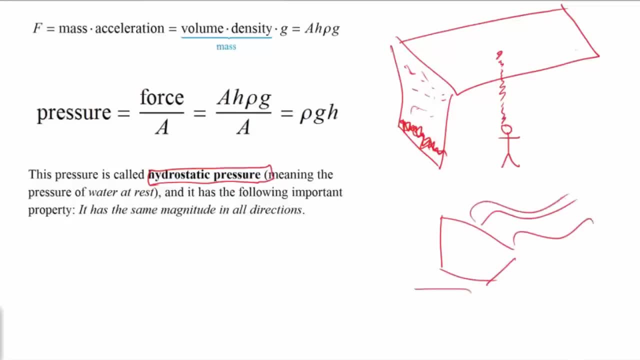 river behind it. Here's your lake at the bottom. All that water is leaning against that dam, and so that's a lot of hydrostatic pressure. So here we can see that we know force is mass times acceleration, and mass is volume times, density times, gravity. 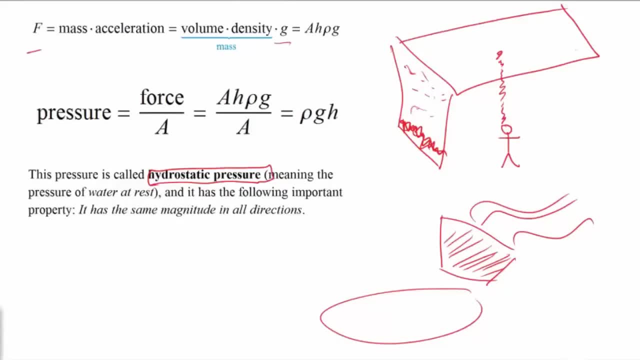 Our total force here is the area times the height, times rho. that's your density times gravity is our volume we're getting by a slice times its height. And then the pressure part is defined to be the force divided by the area. So if we divide by area, we're left with just the density, the gravity and the height. 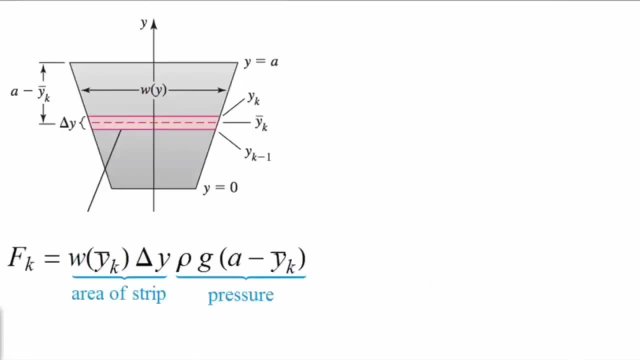 So let's look at a problem that would be like this: Okay, so here again, the force is the area of the strip, so there is okay. so then the total force we're looking for is the area of the strip times the pressure. So pressure is what we just talked about on the last page. 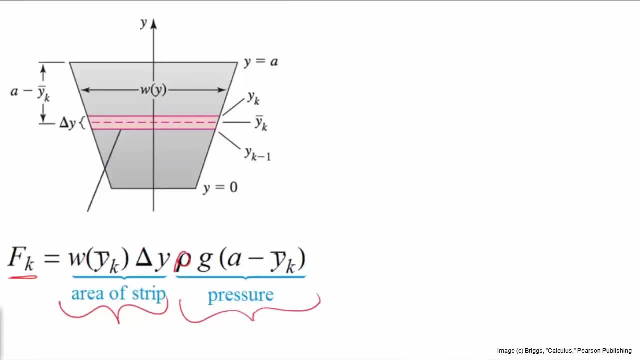 Density, that's going to be a constant. gravity, that's going to be a constant. and then this is the distance, the height, this is how far it is under the water. So this is the top here of your dam. then that's the number A, this is your Y value. 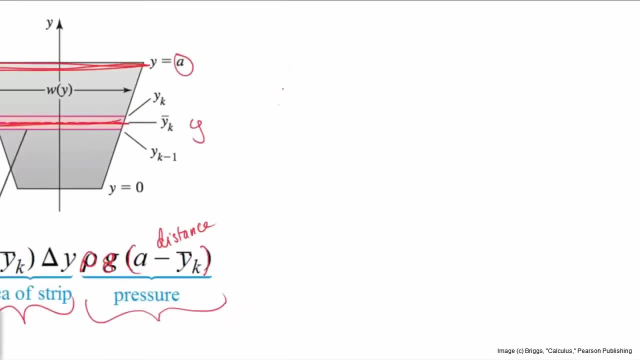 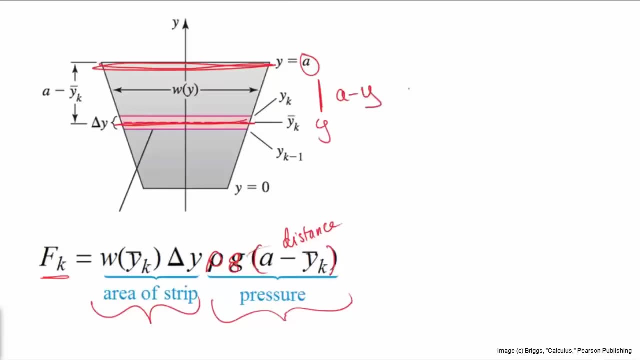 that's the number Y, that distance between them, just like in the previous problem, that distance, The distance is A minus Y. so that's what they're saying here, And then the area of this little strip of water, that area is all at the same pressure. 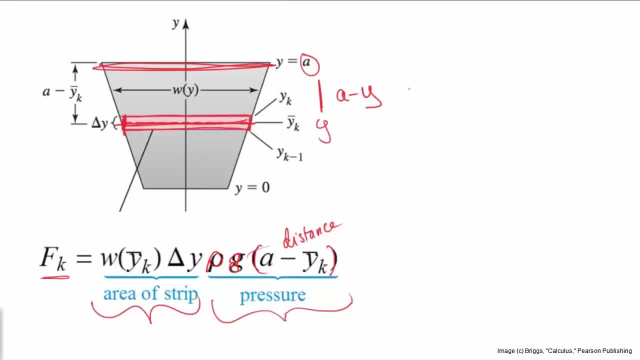 because it's all at the same depth So we can use all of it together. So we need to find the length of the strip and so this W of Y, that's supposed to be that length. they're using W, I think, for width. 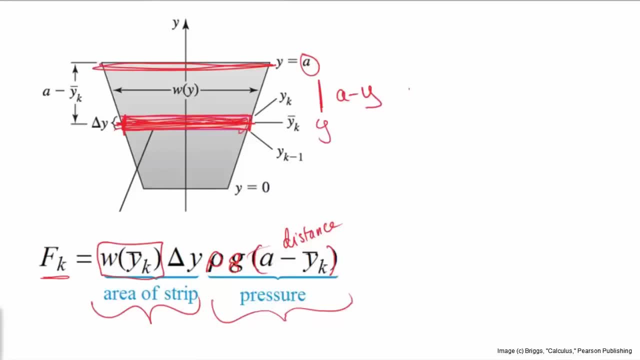 The width of this strip Times the delta Y. the delta Y is how thick the strip is, And if you put all of those together, that's going to give you your force. So here let's try a problem. oh, this is the same thing we just said again, only they're. 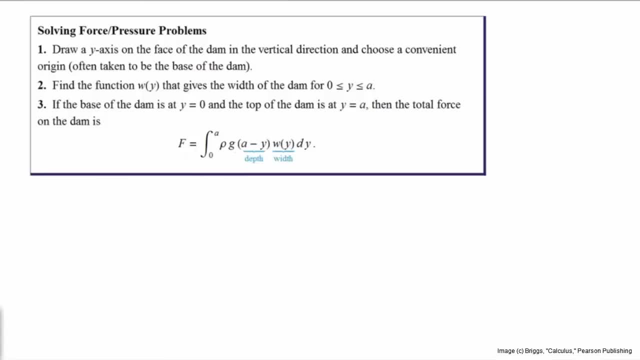 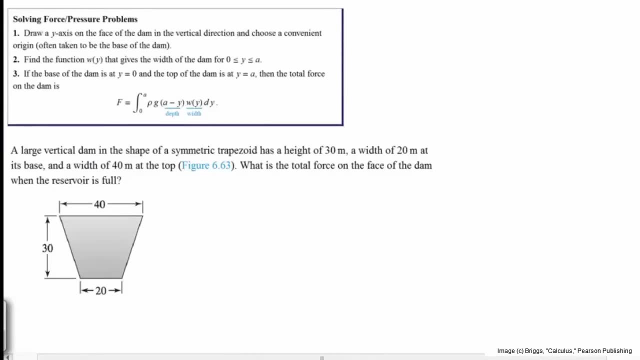 saying you can add up all those little strips, it turns into the integral. Okay, so we have a large vertical dam in the shape of a symmetric trapezoid that has a height of 30 meters, a width of 20 meters at the base. 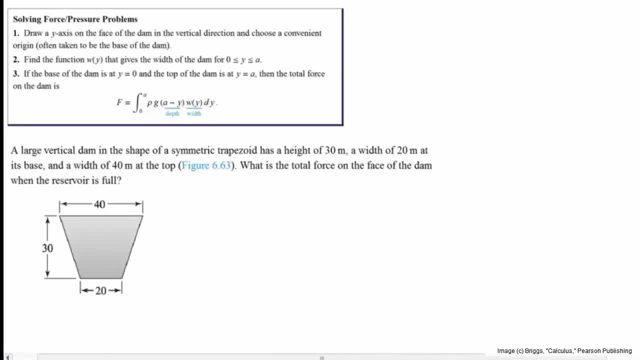 And a width of 40 meters at the top, And what is the total force on the face of the dam when the reservoir is full? So, using this formula they give us, it's going to be the integral, so let's put a: Y is going. 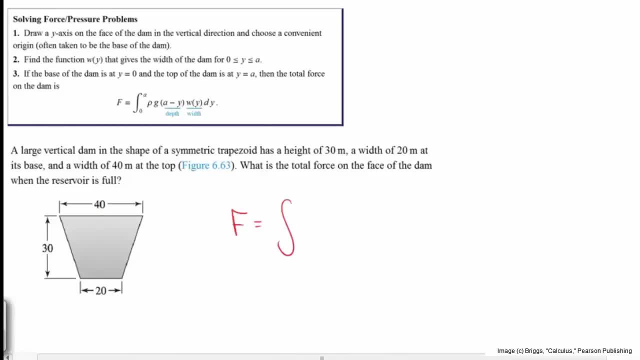 to be our up and down here. so this way is Y. So here's a slice. This distance is going to be Y, So Y is going to start at zero and it's going to go up to 30, right there. 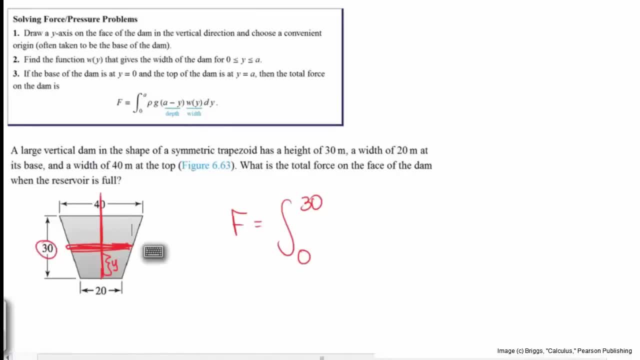 Okay, so now we need our density. that's rho And we'll use from the previous problem. water has a density of a thousand. We need our gravity, that's 9.8 when we're in the metric system. We need our depth. 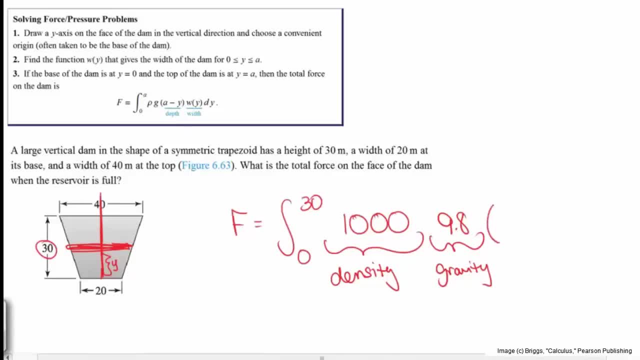 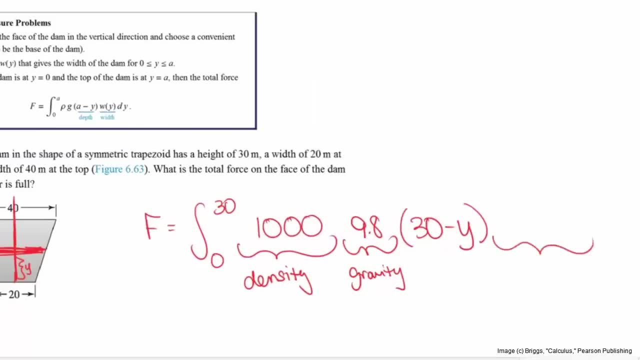 So that is the total depth: 30, minus Y. And then the last thing we need here- this is depth. the last thing we need is the width of each rectangle, And then we're going to have DY, that's the height of each rectangle, and so these two. 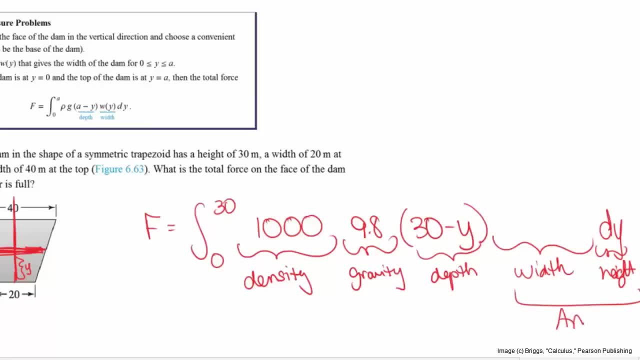 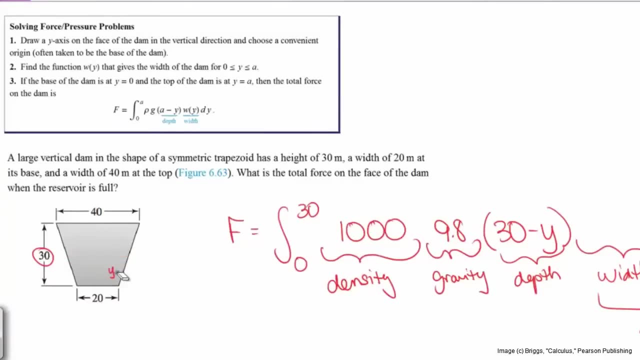 together give you the area. Okay. so how do we find that width? That's the hard part. So we go back to our picture here. We want to find this length right here, And all we know about it is that this distance is Y. 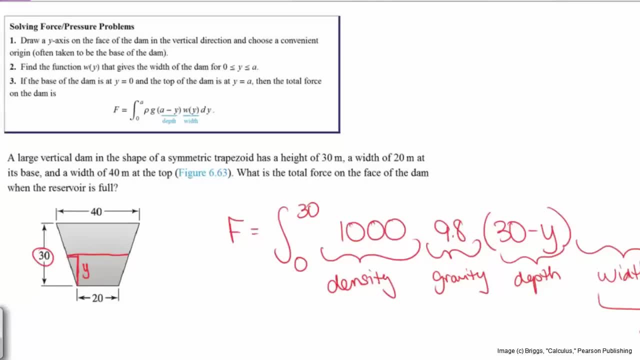 We also know that we could draw a bigger triangle here. Okay, Like this, and we know things about that bigger triangle: This one side, the long side, is 30, and this side- over here we can find that right Because we can split the top up- this is 20,, the total is 40, so this must be 10, and this: 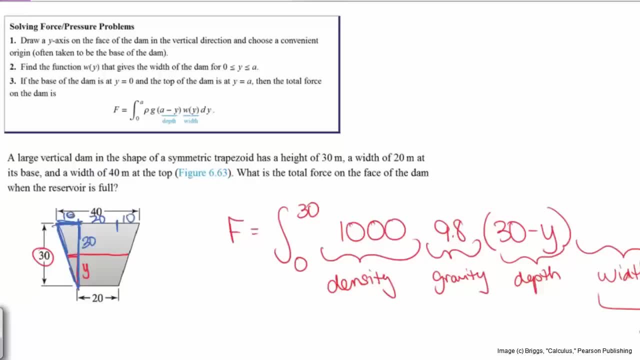 must be 10.. Because it says it's symmetric, it means it's the same on both sides. So we have a big triangle that's 10 by 30, and so our little triangle inside here. this is a similar triangle. You guys remember doing this from related rates. 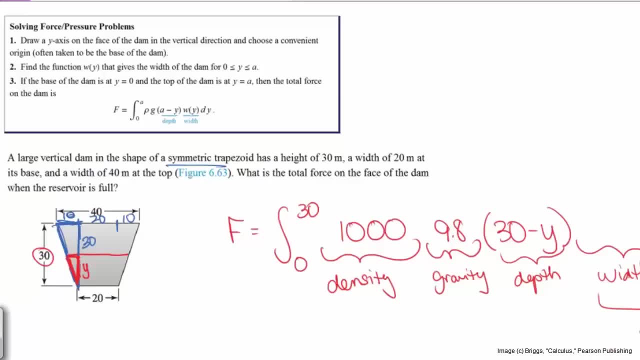 The similar triangle is going to be the thing we want to know by Y. So the thing we want to know divided by Y is just like 10 divided by 30.. So the little piece here that we want to know is one-third Y.